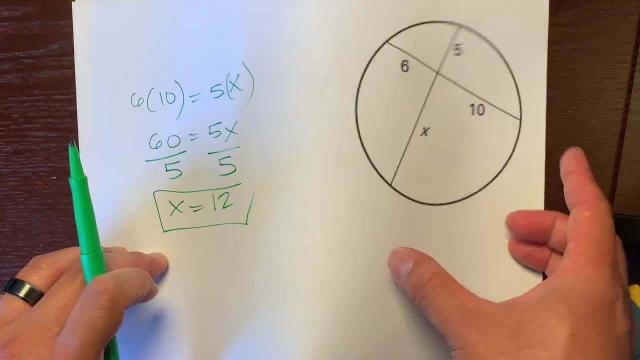 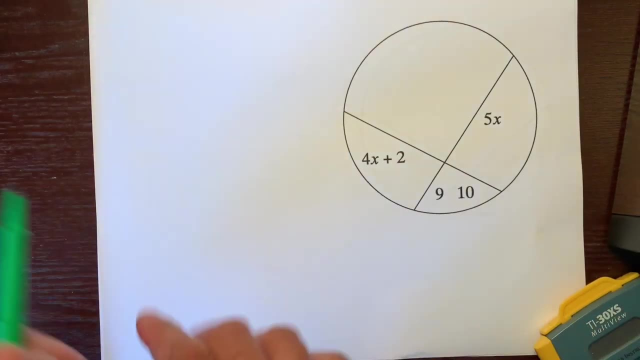 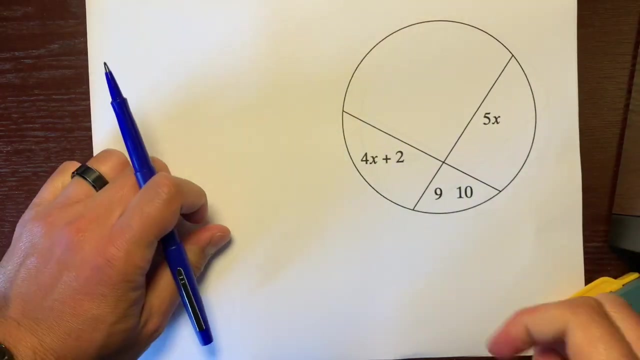 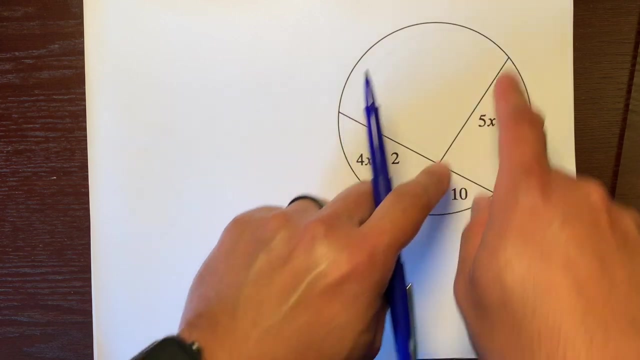 So there's the first example. All right. Second example Might get a little more challenging. Is this one with two x's, two variables? I'll even use another color, just because it's a little more challenging, This blue. So remember it's, you know, two chords that intersect. It's the piece of the one chord times the other piece is equal to a piece of the one chord times the other piece. So 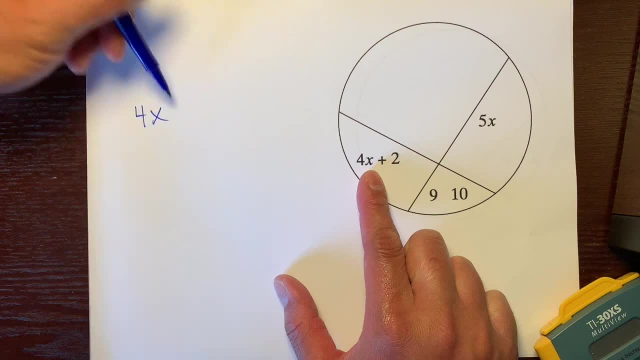 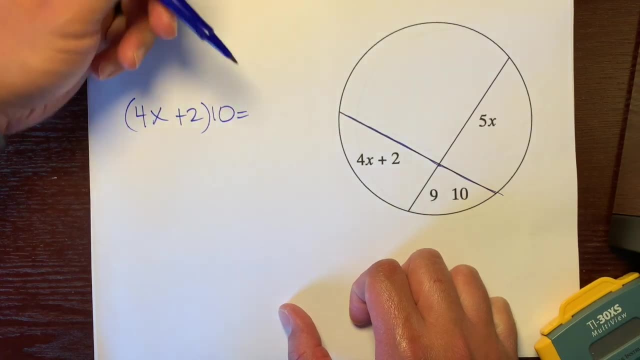 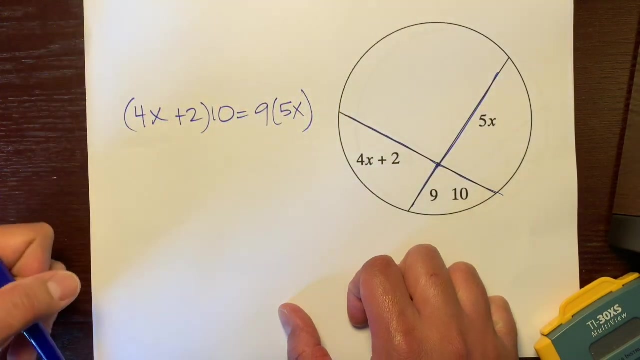 I'm going to write: four x plus two, which is this piece times its other piece, which is ten, Is equal to nine, which is this piece times its other piece, which is five x. All right, So let's just solve this equation. 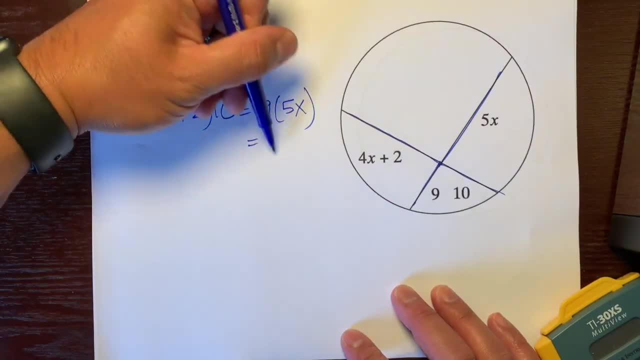 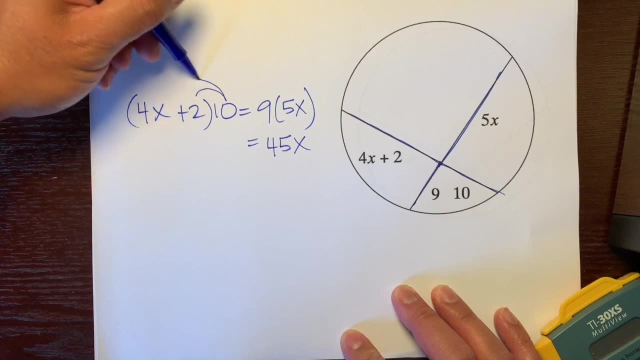 We'll start. on the right side, Nine times five is forty five x, And on this side okay. so we're going to distribute this ten to this two, and this four x 10 times 2 is 20, and then 10 times 4x is 40x. 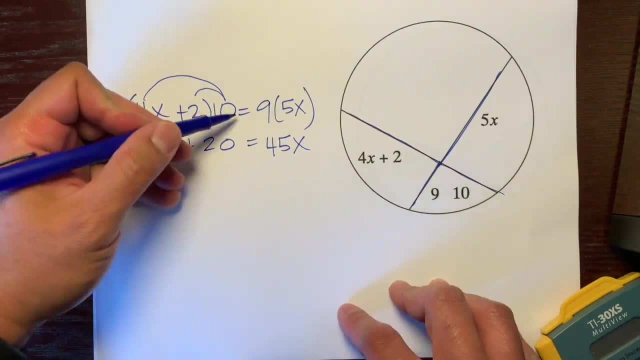 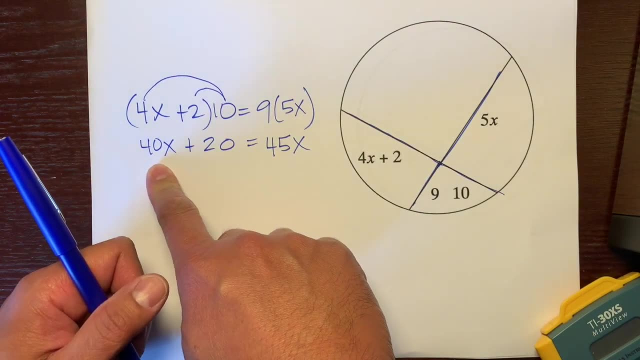 Don't forget to put the plus over there. Don't forget to distribute to both terms inside of the parentheses. Now, let's just solve this. Let's get this 40 to the other side, because this one has an x with it, So let's put all the x's together. 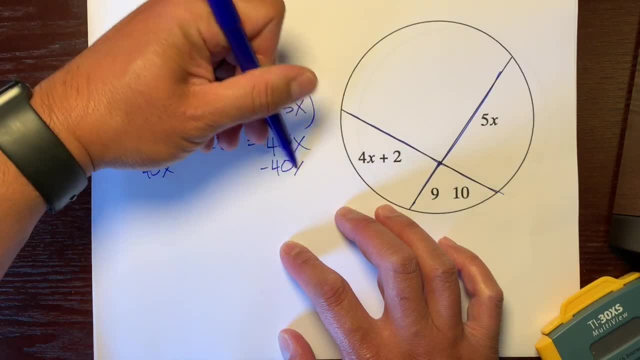 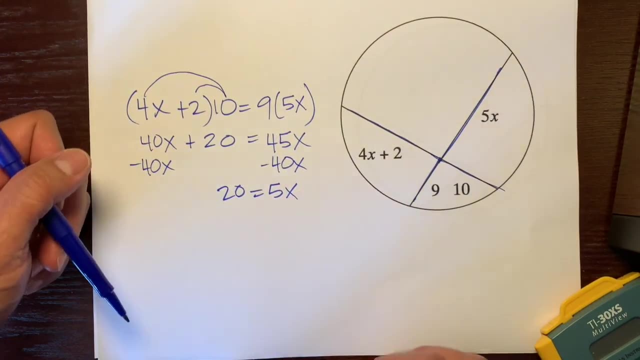 So subtract the 40 here and here, 45x minus 40x is 5x, is equal to 20.. And this is 5 times x. Opposite of multiplication is division. 20 divided by 5 is 4.. 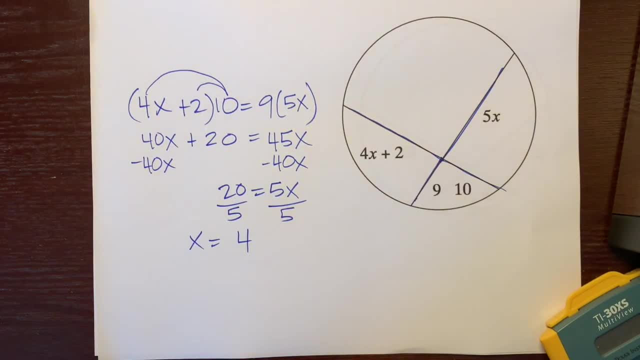 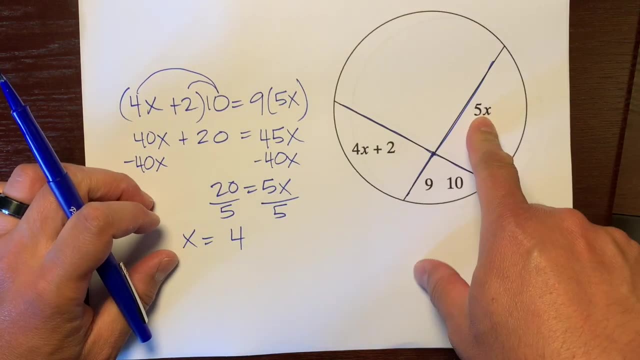 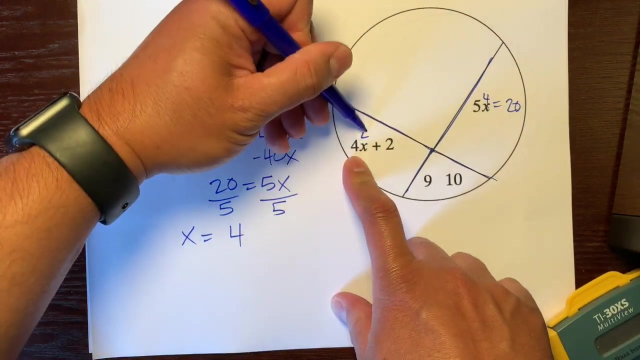 So x is equal to 4.. If you don't believe me, then let's plug it back in. So if we plug this into here 5 times 4. Is 20.. And then, if we plug this into here 4 times 4, is 16 plus 2,, which is 18.. 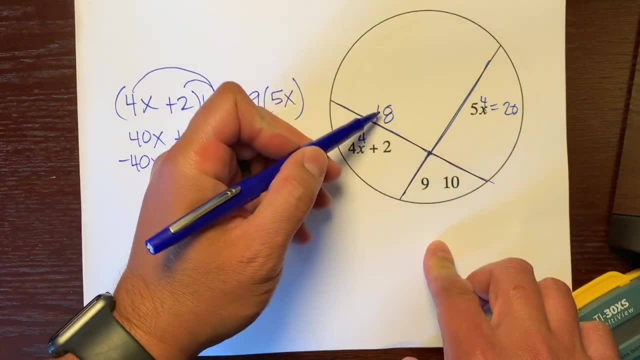 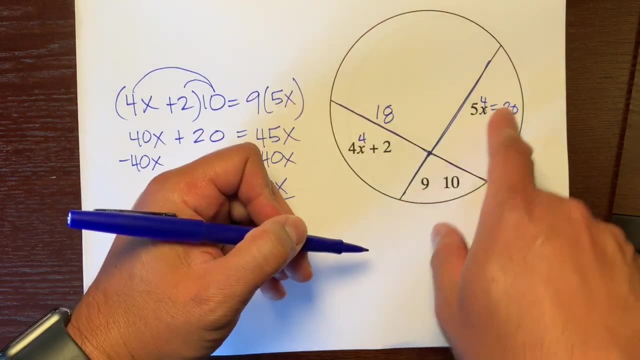 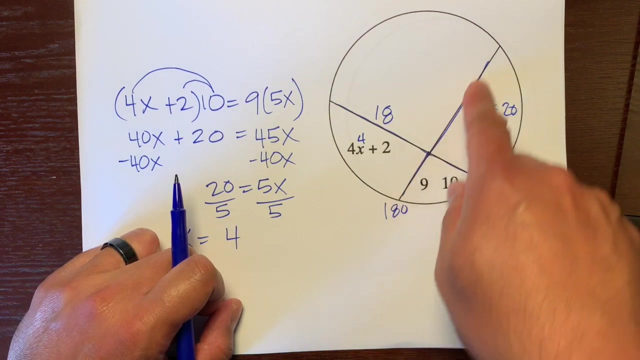 And all these numbers are different. now, But if we multiply this piece times this piece, 18 times 10 is equal to 180.. 9 times 20 is equal to 180.. So that doesn't mean the length This cord is 180.. 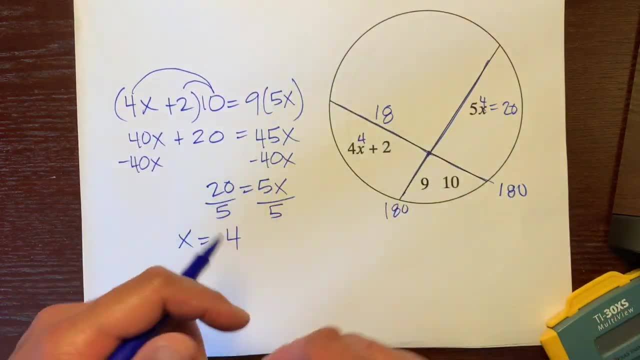 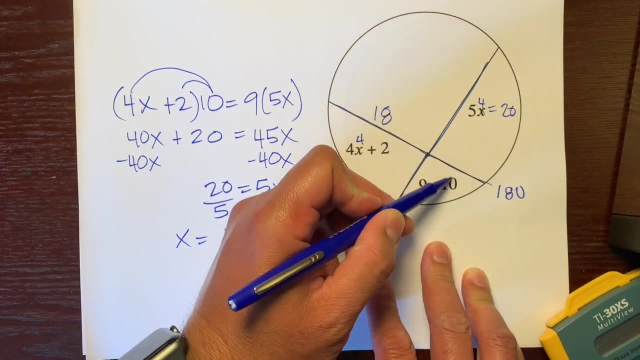 Okay, That just means this piece times. this piece is 180.. Actually, the length of this cord right here is really 18 plus 10,, which is 28.. And the length of this cord is 9 plus 20,, which is 29.. 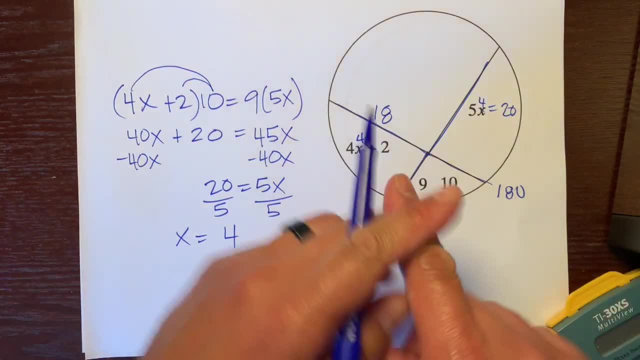 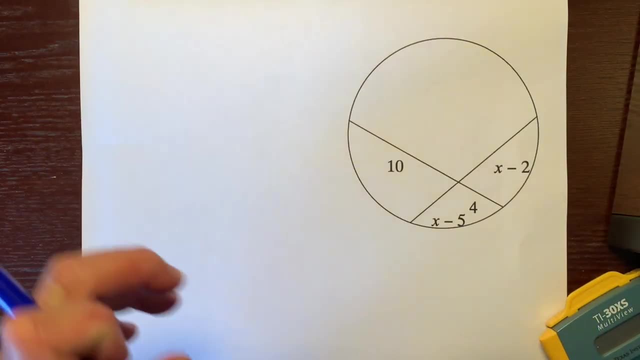 Anyways, the answer here is 4.. You know it's correct, because the products are the same. All right, And the next example, which is the final example. Draw this in your notebooks. I'm going to use a red pen because this is the most challenging out of the three. 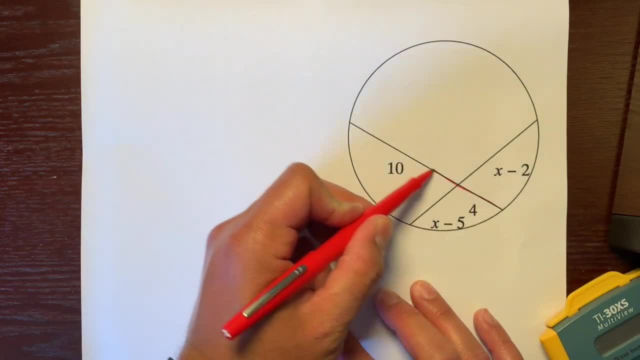 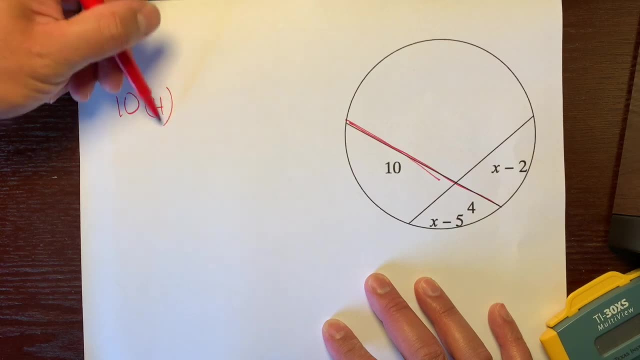 But you've got this, So we're going to start off with this cord right here. So this piece, which is 10 times this piece, which is 4, is equal to now with this cord. Okay, It's, this piece is x minus 5.. 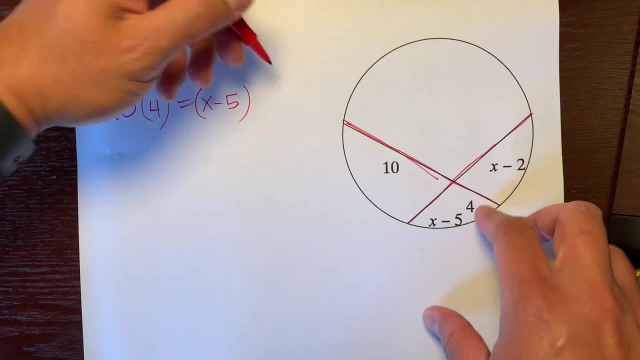 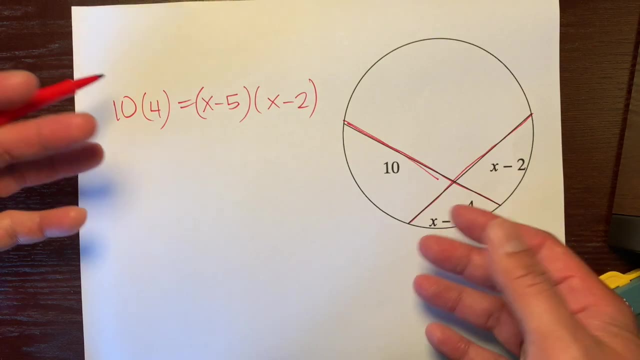 Put a parentheses around that At times, this piece, which is x minus 2.. Put a parentheses around this And you're probably worrying. oh no, this is a lot of algebra. I haven't done algebra in a while, So let's do some algebra review. 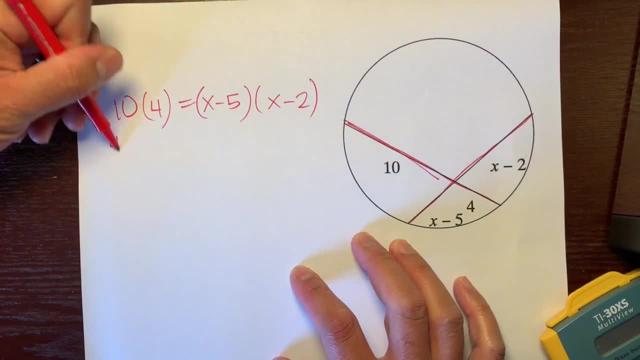 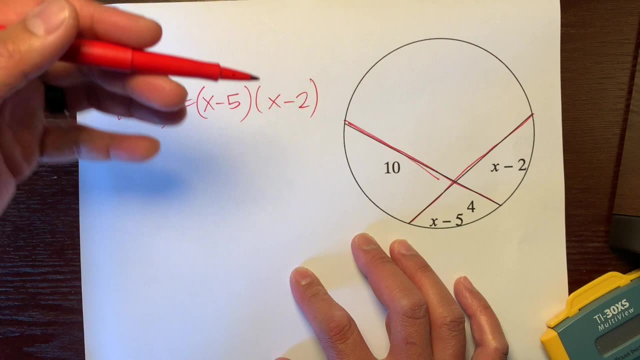 Well, let's do some multiplication review: 10 times 4 is 40 is equal to. Now we're going to distribute twice. Or if you're your friends and your teachers, or whoever your mom, your dad says, use foil, It's the same thing. 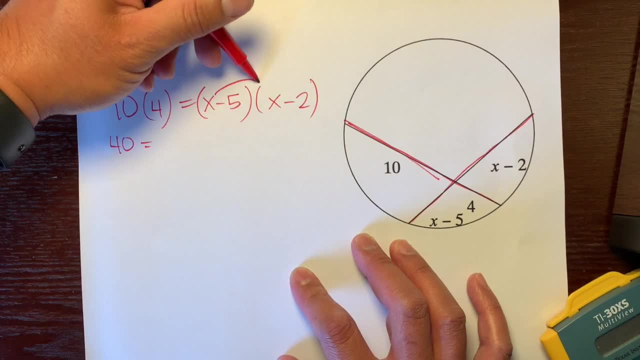 So I like to say: distribute twice. We're going to distribute this x Here and to here, Okay. So that's, we're going to distribute it. So x times x is x squared, Okay. X times negative 2 is negative 2x. 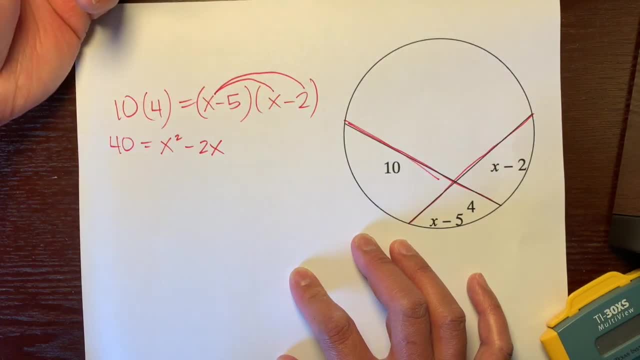 Right there, And then we're going to do distribution again. So we're going to distribute this negative 5 to here and to here. So there we're going to distribute twice. Distribute this x, once X here, Then this negative 5.. 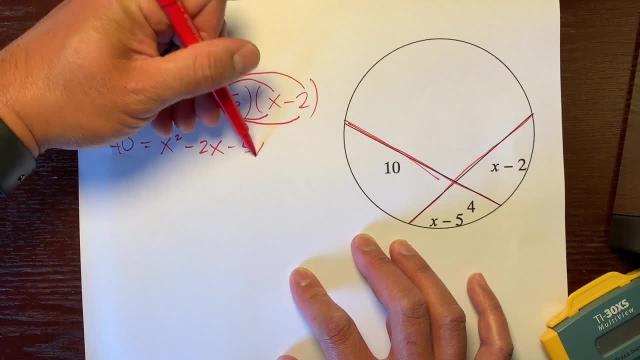 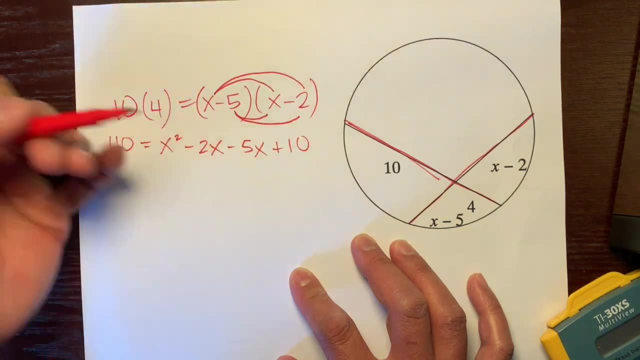 So there's two, So negative 5 times x is negative, 5x Negative 5 times negative: 2. Two negatives make a positive, So plus 10. So there's that, And so let's look at this side. Can we combine any like terms? 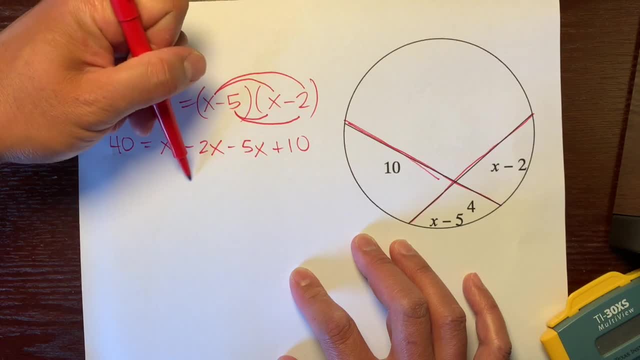 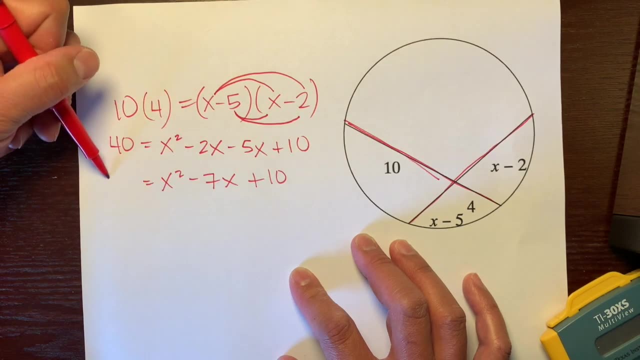 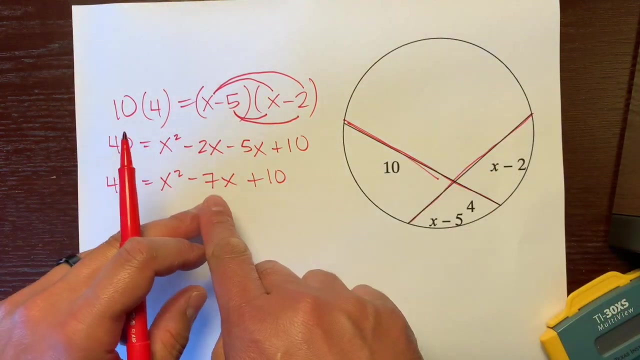 Yeah, we combine these two terms. Negative 2x minus 5x is negative 7x. Bring down that 10.. Bring down that x squared And bring down that 40.. So now we have all this algebra. goodness, We want to make this. 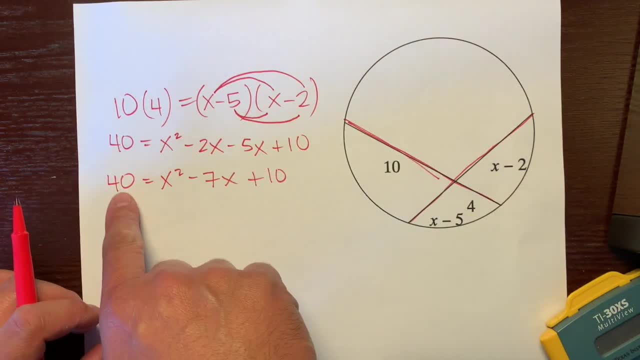 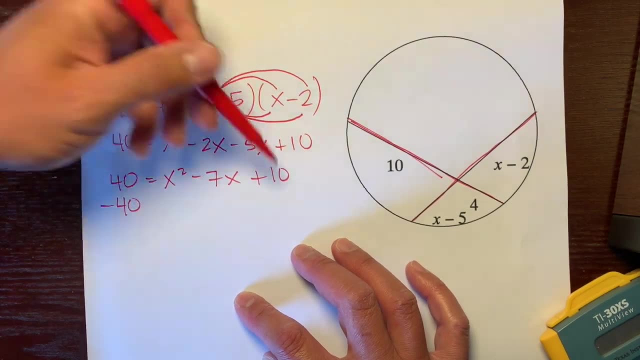 Entire equation equal to 0.. How do we make that equal to 0?? Well, we'll make this. The easiest way is to get rid of this 40. And bring it to the other side. So subtract it. So here and here. 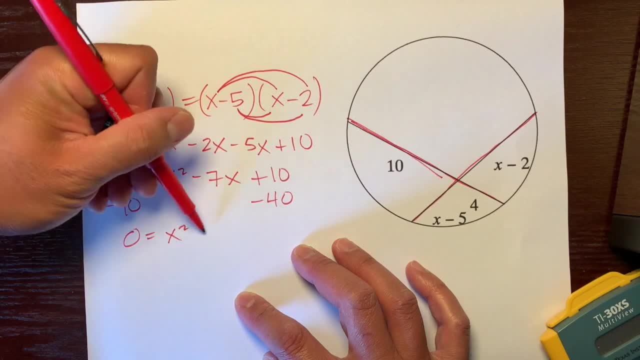 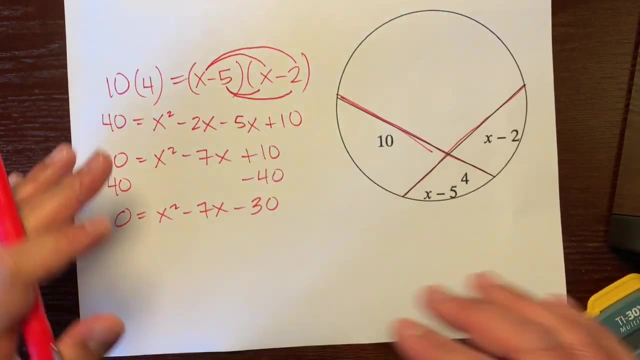 And 40 minus 40 is 0.. Is equal to x squared minus 7x, And 10 minus 40 is negative 30. So now that we have it, equal to 0.. We're going to factor it So. 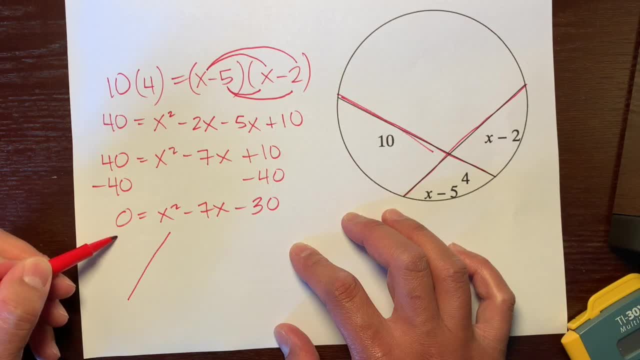 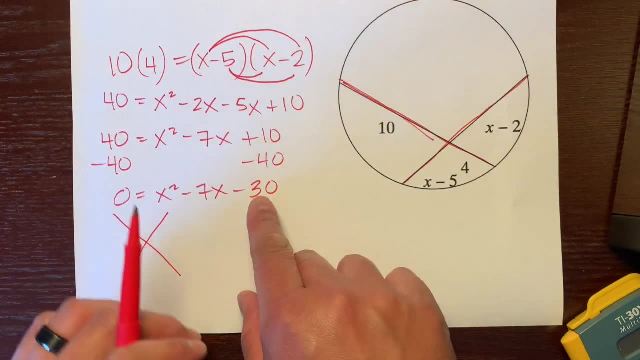 If you remember your Algebra 1 teacher last year, They may have showed you this. If they didn't, Sorry, I'm going to show you this now, So hopefully it'll be quick for you. So we need two numbers that multiply to the C. 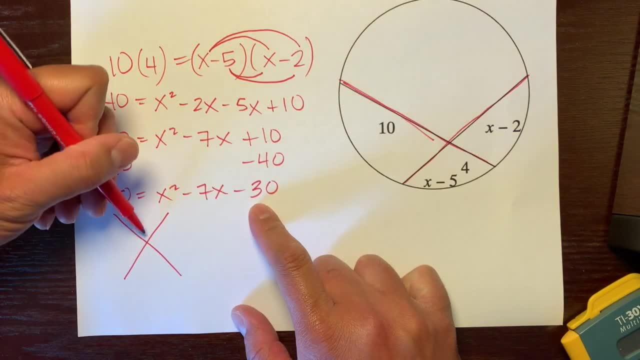 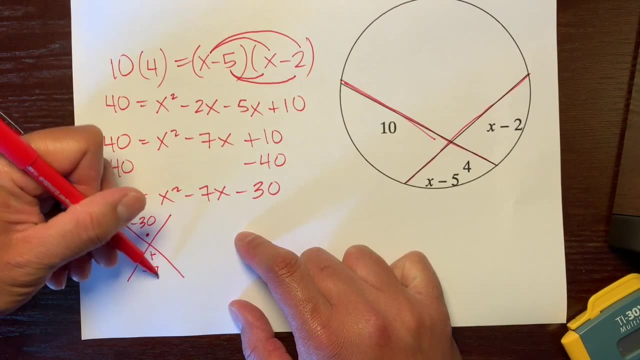 So this is A, B and this is the C term. So we want two numbers that multiply to this negative 30. And two numbers that add up to that negative 7. What multiplies to negative 30? 5 and 6.. 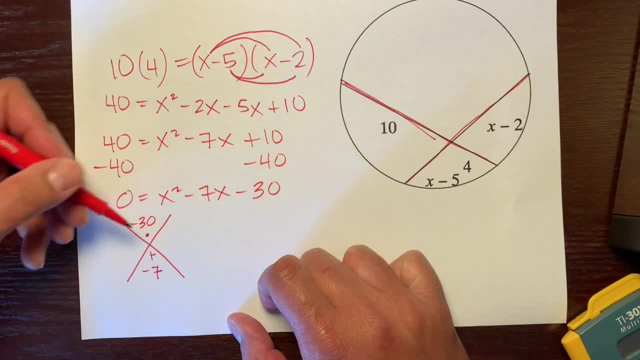 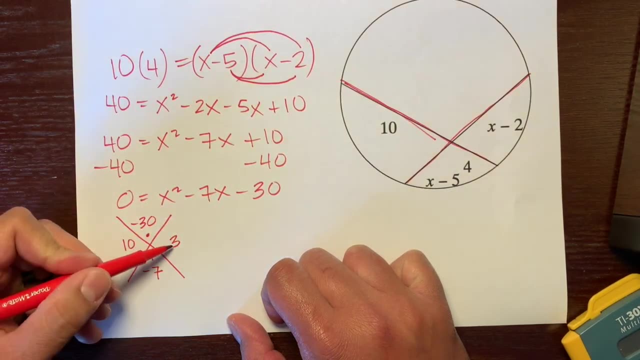 But those one add up to 7.. Let's, how about 30? For negative 30,, how about 10 and 3?? Well, those two multiply to positive 30. But we want them to multiply to negative 30.. 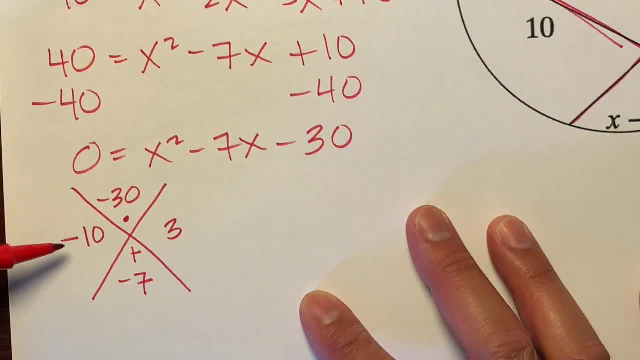 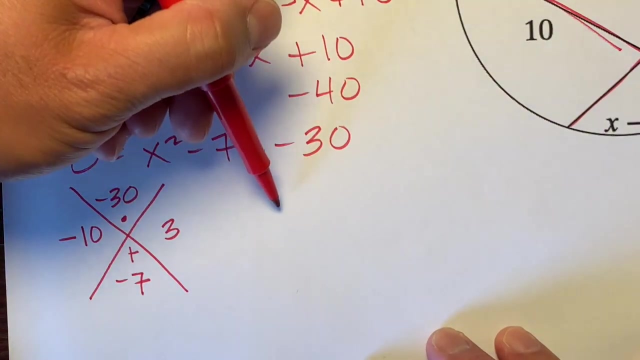 So what if we made this into a negative 10? Negative 10 times 3 is negative 30. And well, does it work? Yeah, negative 10 plus 3 is equal to negative 7.. So, yes, So what we're going to do is we're going to take our two numbers. 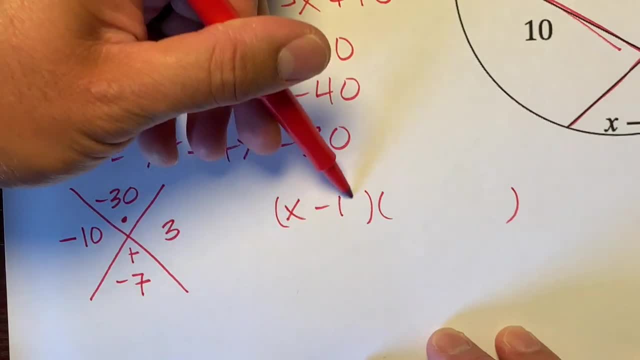 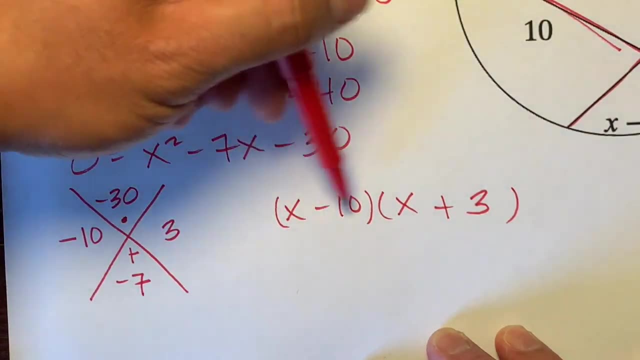 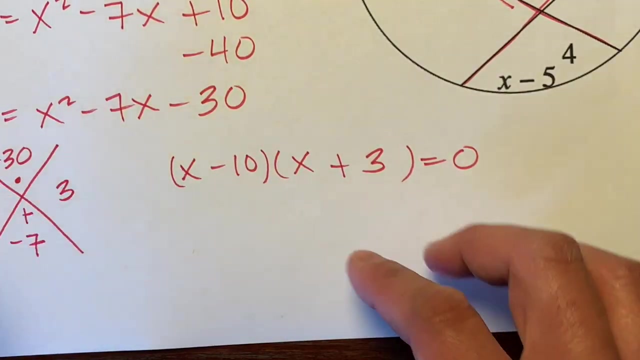 So now we're going to put these two numbers into parentheses, So we're going to write x minus 10 and x plus 3.. And then, since this equals 0, we're going to set this equation equal to 0.. And we're going to use a zero product property. 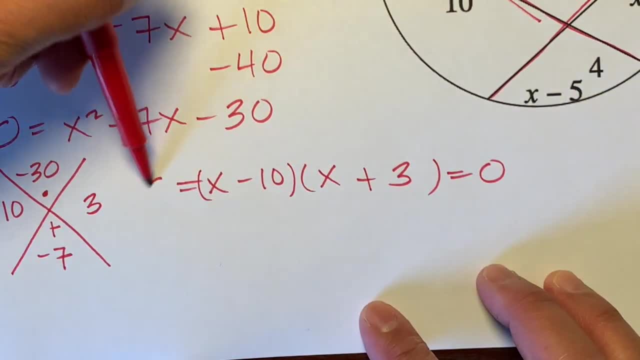 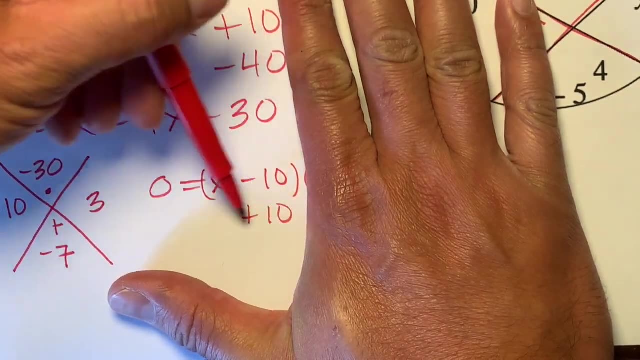 When you use a zero product property, you just set both parentheses equal to 0 and solve for them: x minus 10 is equal to 0.. How do we get x by itself? We're going to add the 10 to both sides. 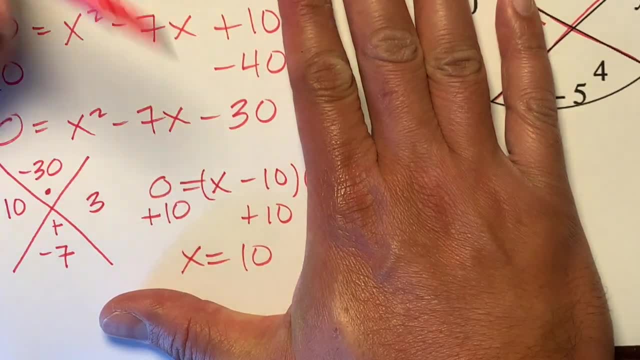 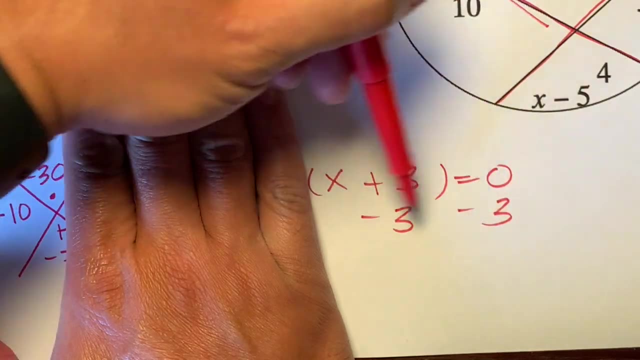 So x equals 10.. So there's our first answer, And now we'll focus on this one. for the zero product property, x plus 3 is equal to 0.. We'll subtract 3 from both sides, So x is equal to negative 3.. 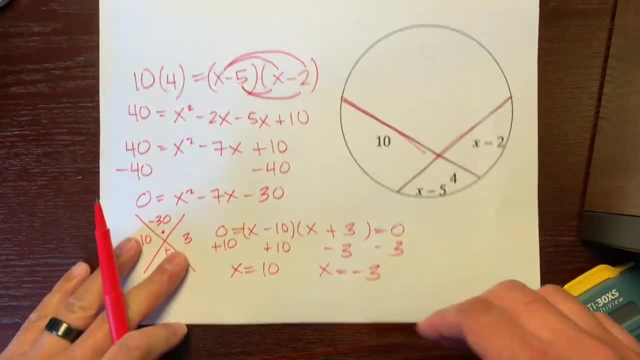 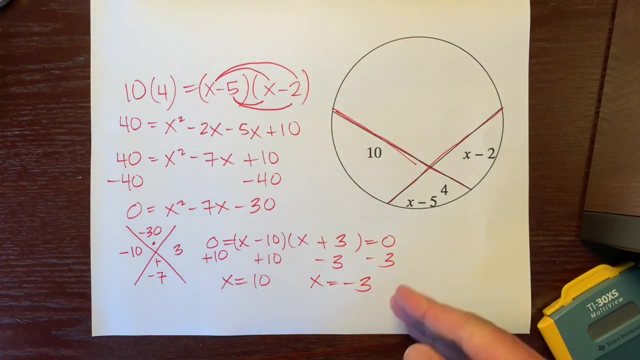 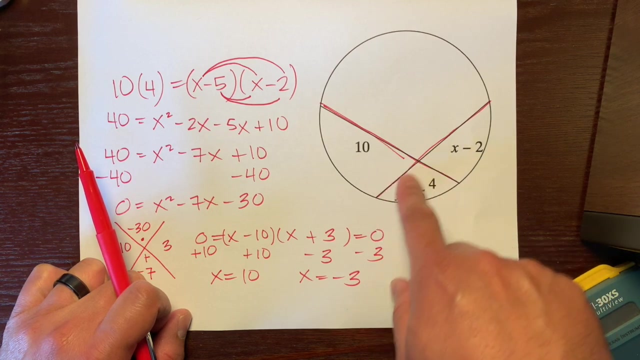 So now we've got x by itself, We've isolated x, But don't box both of these yet. OK, Both of these will work. So let's do this If we plugged in this 10 into here for this segment, right here. 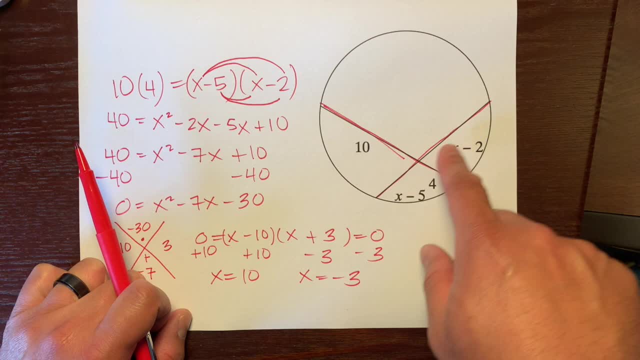 so 10 minus 5 would be a positive 5.. If we plugged in the 10 here, 10 minus 2 would be a positive 8.. So that's fine, because it's all right. So 10 minus 5 would be 5.. 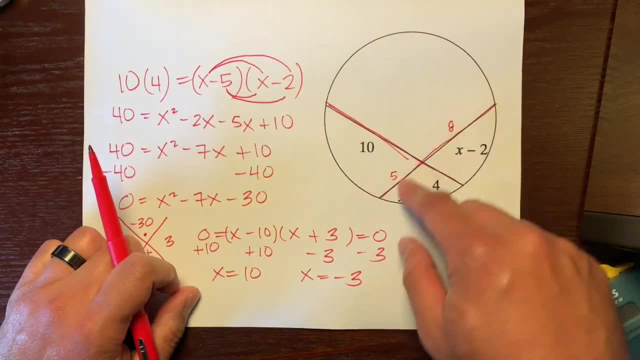 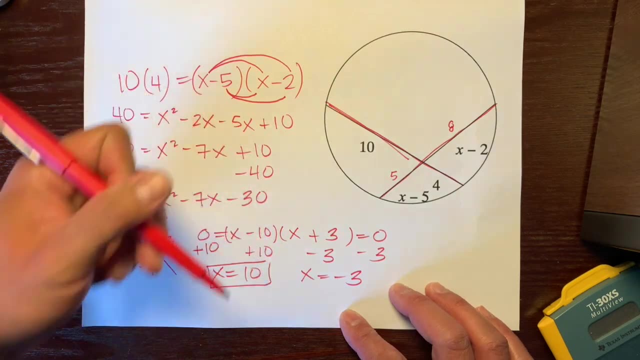 10 minus 2 would be 8.. OK, We multiply these 8 times 5 is 40.. 4 times 10 is 40.. So their products are the same. So I'm going to box this. But here's the thing with this negative right here. 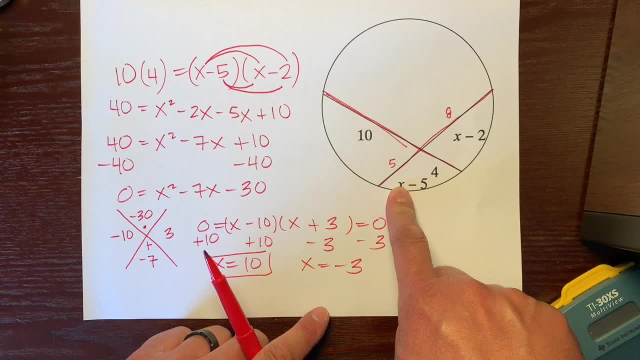 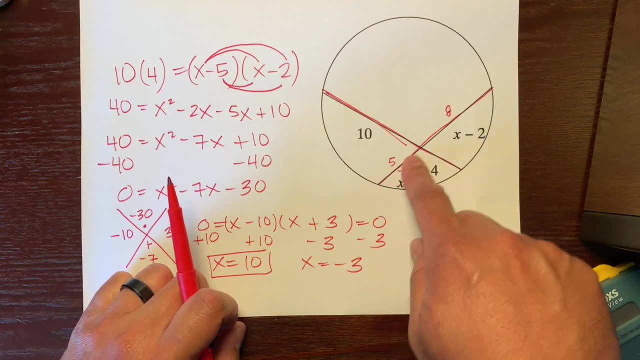 If I plugged in this negative into here, negative 3 minus 5 would be negative 8.. I'm just going to stop right there. I'm not even going to plug in that negative 3 in here, because a chord or anything of length cannot be a negative length. 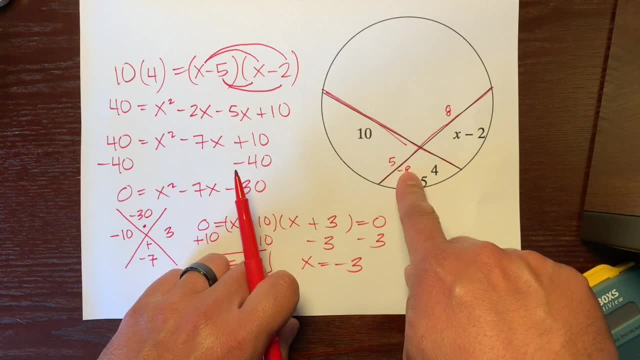 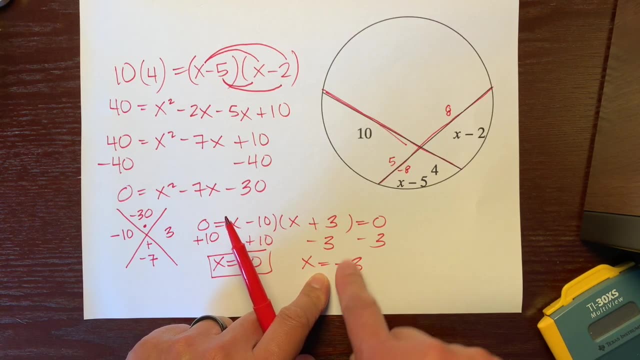 So if we plugged in this negative 3 in here, this would give us a negative length. So yeah, even though we did all this work, an X by itself, because this negative value gives us a negative length, we can't use this value on that. 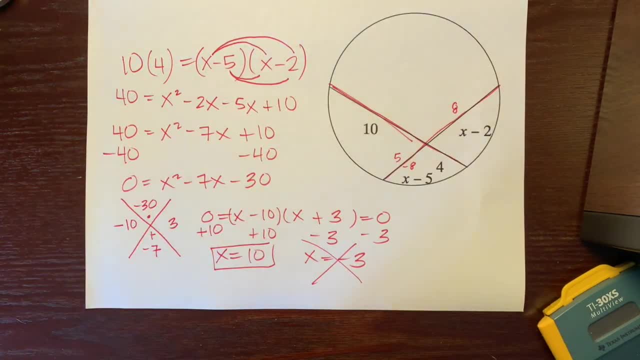 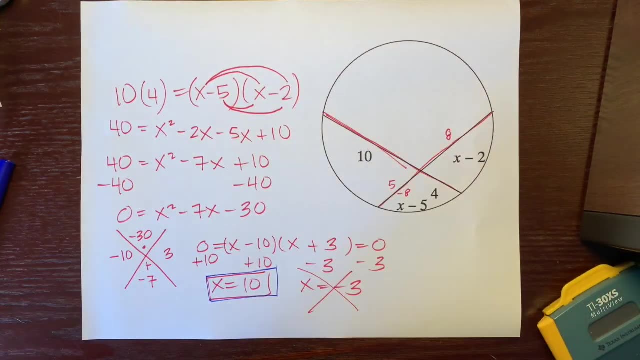 So this is our one and only answer. X is equal to 10.. So that's how you use the intersecting chords theorem And that's how you do some algebra with factoring And that's how you get the answer. Hope it helps. Have a great day, Bye.